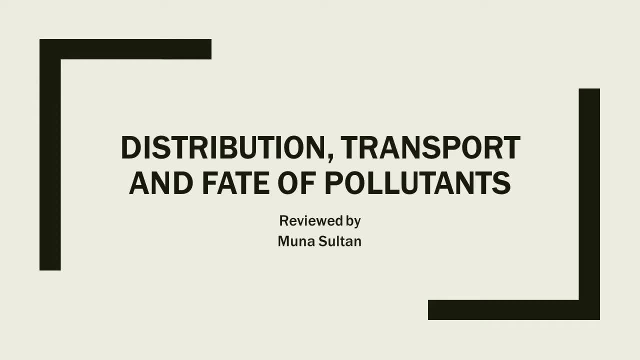 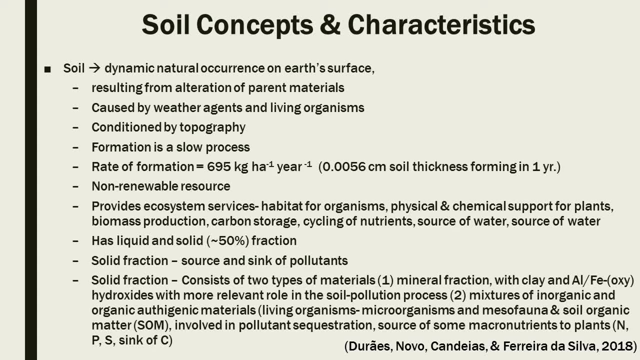 Distribution, Transport and Fate of Pollutants. Reviewed by Mina Sultan. Soil is a dynamic natural occurrence on Earth's surface from the alteration of parent materials caused by weather agents in living organisms and conditioned by topography. Soil is composed by a liquid and gaseous fraction, where the solid fraction is about 50% of the. 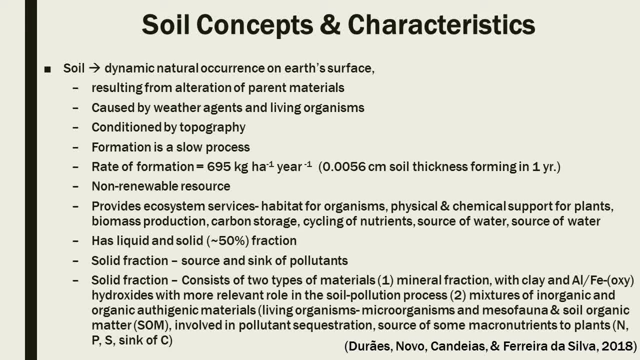 soil constituents in a source and sink of pollution. Two types of solid materials constitute this fraction: a mineral fraction where clay minerals and L-slash-Pha-Oxy hydroxides relevant role in the soil pollution process. The second fraction, organic, is a main source of some 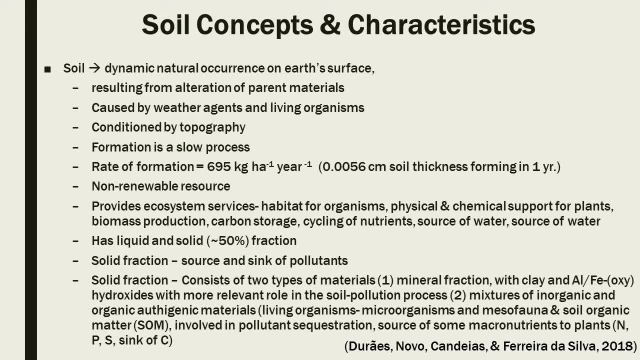 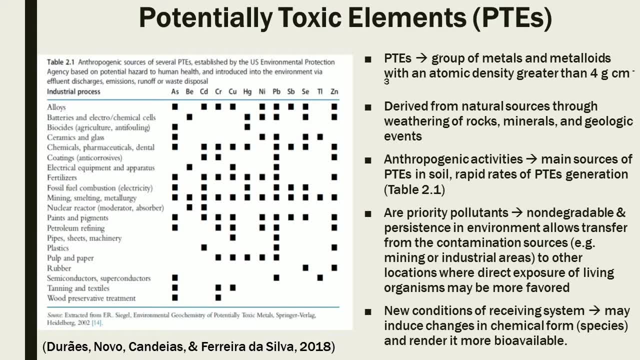 macronutrients to plants, a sink of carbon, and it is actively involved in pollutants sequestration. Soil pollutants can be divided into two main groups: the organic pollutants and the inorganic pollutants. An example of inorganic pollutants is a mixture of organic and inorganic pollutants. 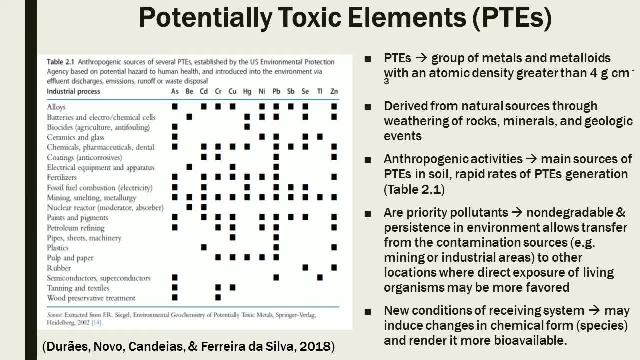 The two is potentially toxic element and both can have natural or anthropogenic origins. May experience increased or decreased availability over time due to their form and changes in physicochemical conditions in soil. The availability of opps tends to decrease over time and is closely related to their 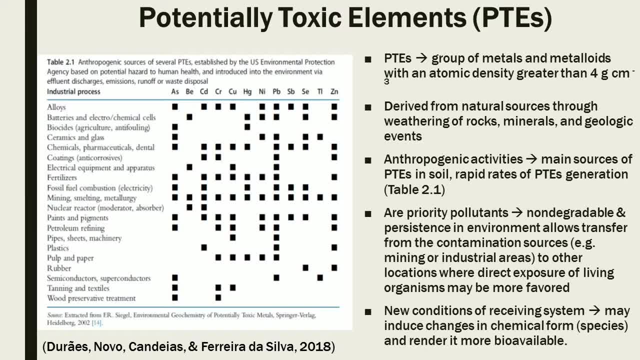 degradation, where they are decomposed into simple units or functional groups of lowest toxicity. Table 2.1 lists anthropogenic sources of several PtoE4.. The original and used in the meantime by PtoE4, linked to a soil, The soil pollution. 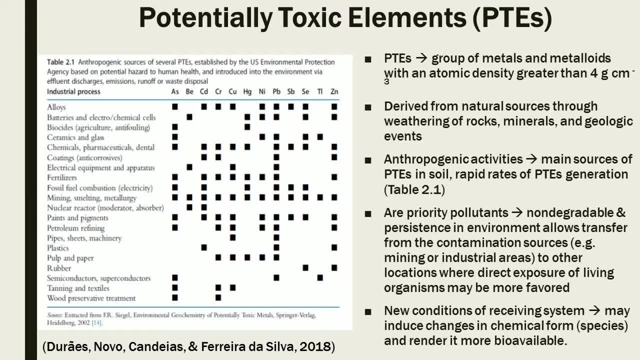 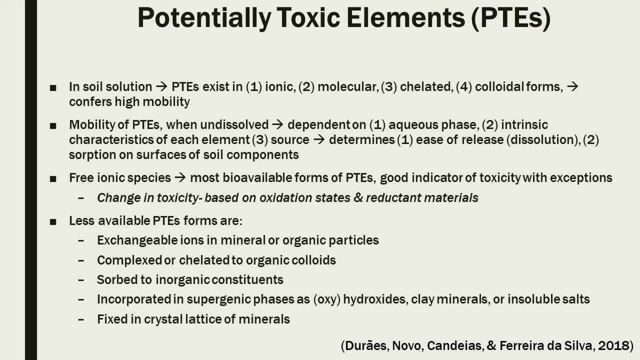 from the industrial front In soil system. PTES can occur in the soil solution under ionic, molecular, chelated and colloidal forms, conferring them high mobility, or associated with the solid fractions. Thus, from the ready to less available, PTES forms are. 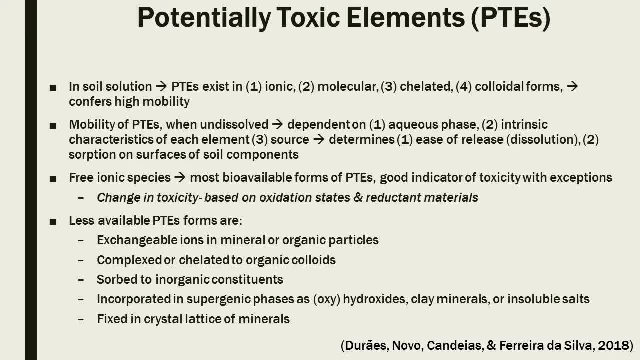 1. Exchangeable ions in mineral or organic particles. 2. Complex or chelated to organic colloids. 3. Sorb to inorganic constituents. 4. Incorporated in supergenic phases as oxy, hydroxides, clay, minerals or insoluble salts. 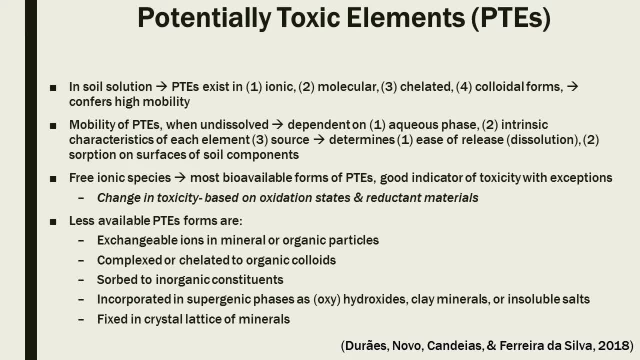 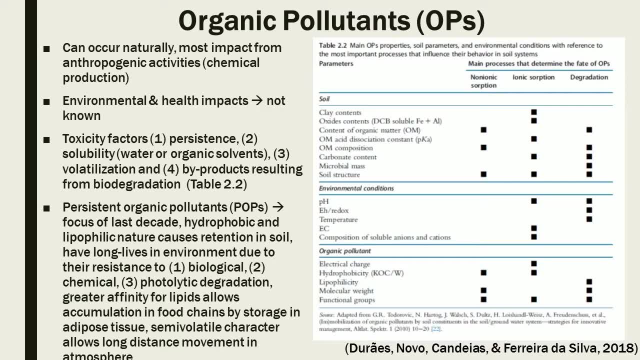 And 5. Fixed in crystal lattice of the minerals. Ops can occur naturally or from anthropogenic sources, such as production of chemical compounds. For many of these chemicals, the environmental and health impacts are not even known. The most important factors regarding ops toxicity are: 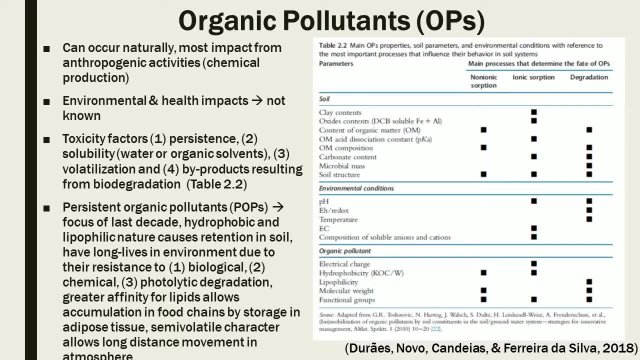 1. Persistence, 2. Solubility, 3. Volatilization and the by-products resulting from their biodegradation. Table 2.2 summarizes the main properties that control the behavior of ops and various soil processes that determine the fate of organic pollutants. 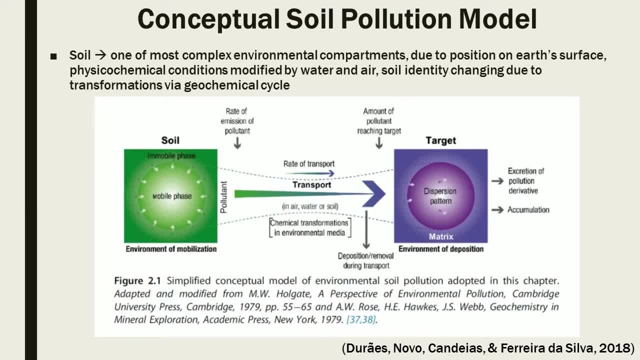 Soil is one of the most complex environmental compartments, where this complexity arises from its position on the Earth's surface. Soil identity is changing as it passes through the major transformations of a geochemical cycle, by the redistribution, fractionation and mixing of its constituents with other. 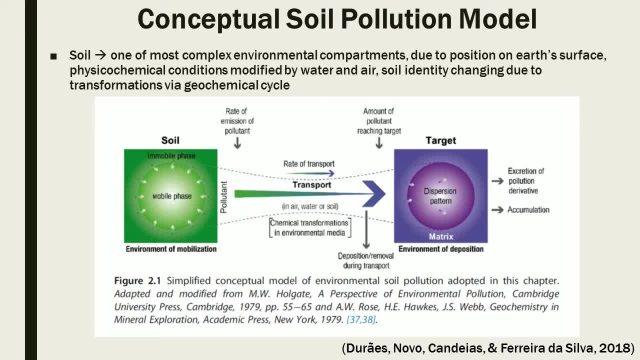 materials and pollutants. Figure 2.1 is a conceptual soil pollution model created using the CLEAR approach and represents the overall cycling of pollutant in the soil system. Factors that affect soil pollutants' distribution, transport and fate are physical and chemical. Soil identity is changing as it passes through the major transformations of a geochemical cycle. 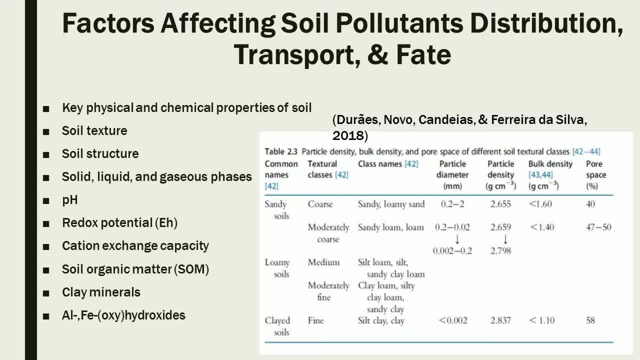 by the redistribution, fractionation and mixing of its constituents with other materials and pollutants. Soil identity is changing as it passes through the major transformations of a geochemical cycle by the redistribution, fractionation and mixing of its constituents with other materials and pollutants. 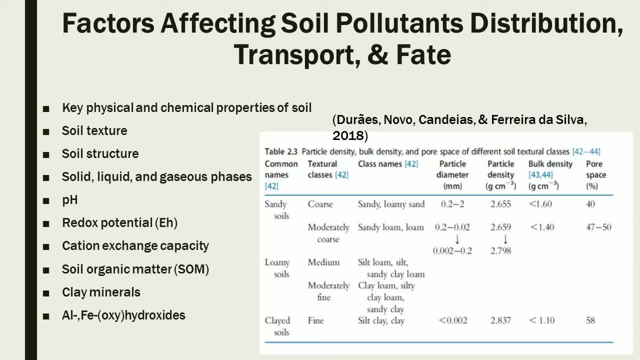 Soil identity is changing as it passes through the major transformations of a geochemical cycle by the redistribution, fractionation and meeting of its constituents with other materials and pollutants. Factors that affect soil, pollutants' distribution, transport and fate are physical and chemical properties of soils, soil texture, soil structure, the solid-liquid and gaseous phases. 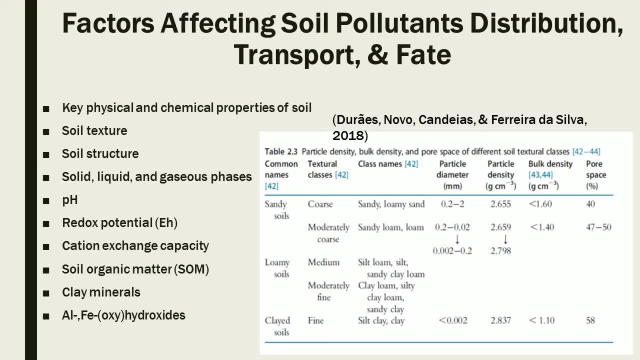 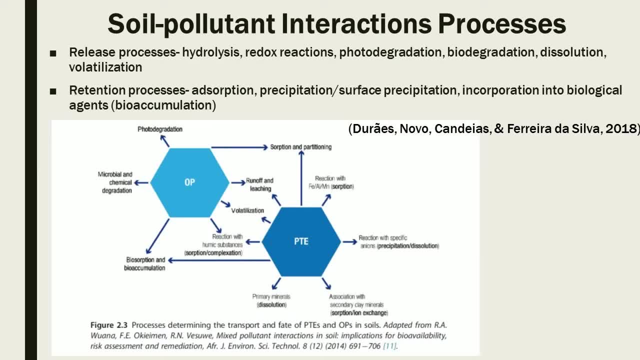 caddion exchange capacity, soil, organic matter, clay, minerals and alpha-oxy hydroxides. The main processes that will determine the root of a pollutant in soil are those: 1. promoting the release of the contaminant from a specific soil matrix. and. 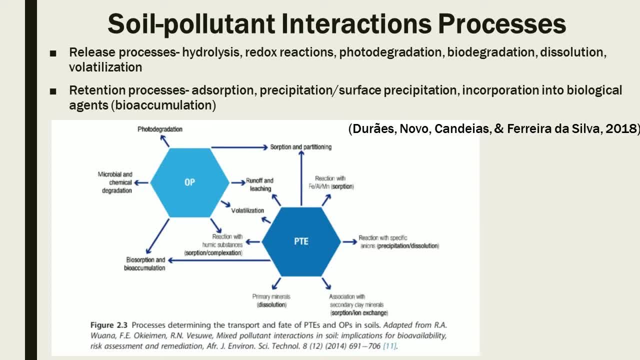 2. occurring between the pollutants and the soil components, where interaction will allow pollutants migration or retention in soil. The release of a pollutant by transformation of the soil matrices is dependent on hydrolysis, redox reactions, photodegradation, biodegradation, dissolution and volatilization.